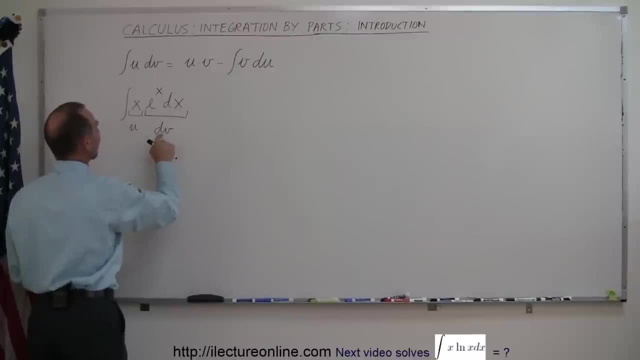 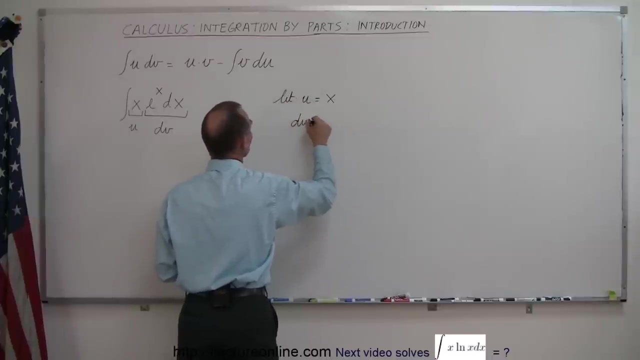 portion right here represent dv, because I can take dv and easily integrate it to v, because integral of e to the xdx is simply e to the x. If I then do the following thing: I let u equals x, dv equals dx. If I take the differential of both sides, I get du is equal to dx. and then, if I let 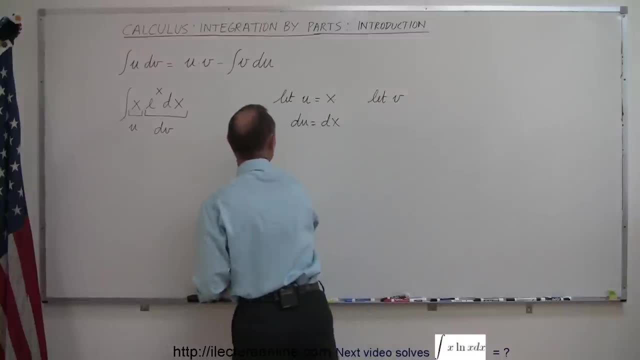 v or not v but dv. if I let dv be equal to e to the xdx, then v, which is the integral of that, would simply be e to the x, without the dx. Of course we do not yet put in the constant of. 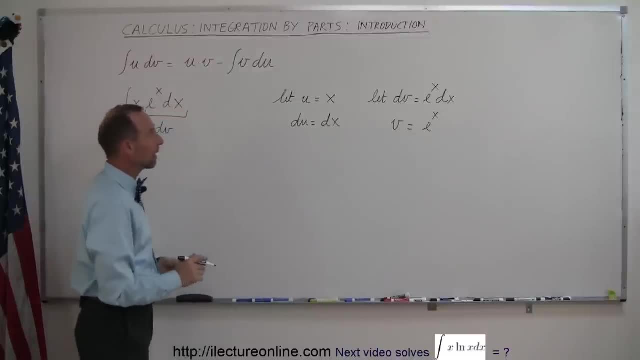 integration. We'll worry about that later. All right, so now I have identified my u and my du, my dv and v. substitute those things back into my equation like this, So I can then say that this integral is equal to u, which is equal to x. right here times v, which is equal to e, to the x. 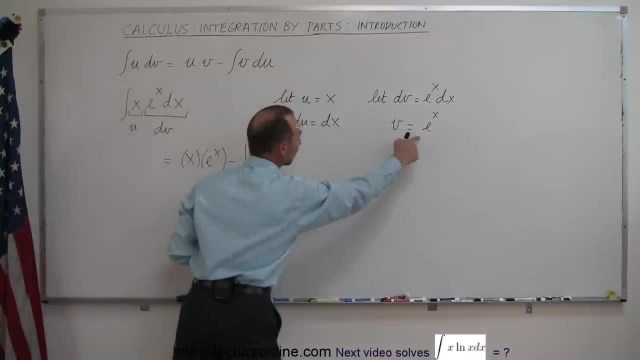 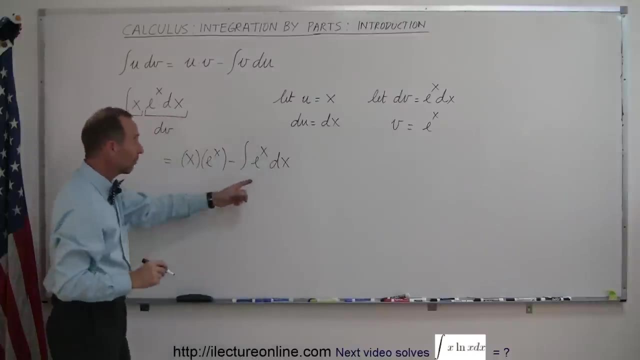 minus the integral of v and v is e to the x times du, which I determined to be dx And now notice that this is a very easy integral to integrate And I can now write this as x times e to the x minus dx. 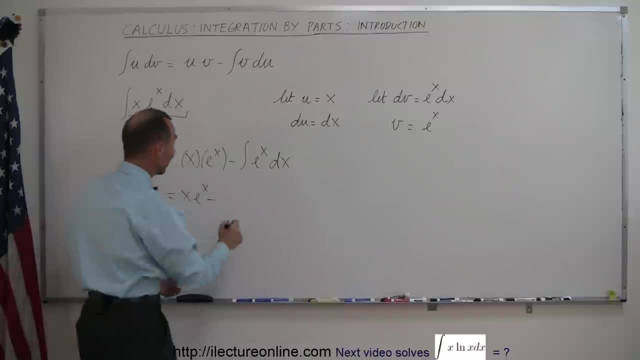 is the integral of e to the x, dx, and of course, the integral of e to the x is e to the x. and of course, don't forget the constant of integration. What we could do at this point is maybe factor an e to the x, and so this could be written as e to the x times x minus 1, plus a constant of. 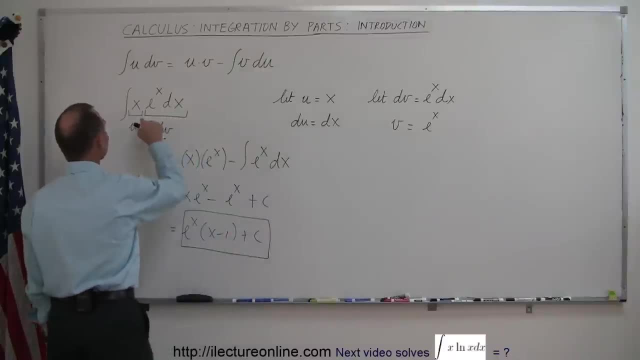 integration and notice. this is the integral of this, and without the method of integration by parts you'd have a hard time figuring that out. So here's a very nice introduction to how you use integration by parts. Now I'll show you a whole bunch of examples in the next videos so you can. 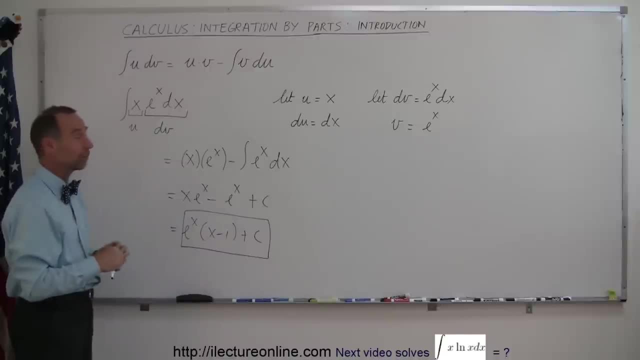 follow and see how that can be applied to a whole array of different kinds of problems and, with certain kinds of tricks which I will show you later as well, you can do some amazing things. so stay tuned, come and watch some of these videos if you're interested in learning how to do integration by parts.